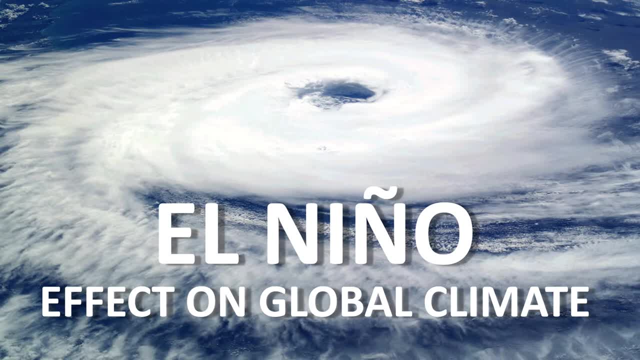 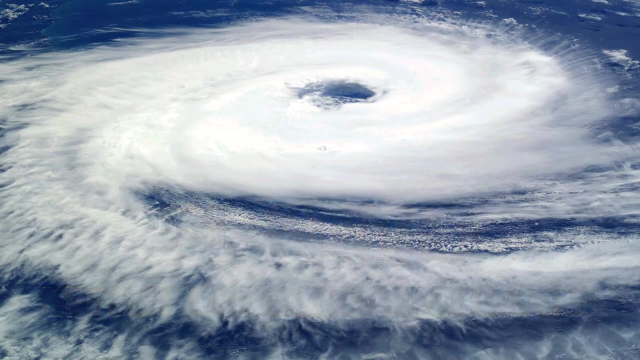 El Nino. What is El Nino and what is the effect on the global climate? El Nino is the warm face of El Nino- Southern Isolation, we call it ENSO- and developed in the central and east-central equatorial Pacific And this event, occurring periodically every five-seven years and affect 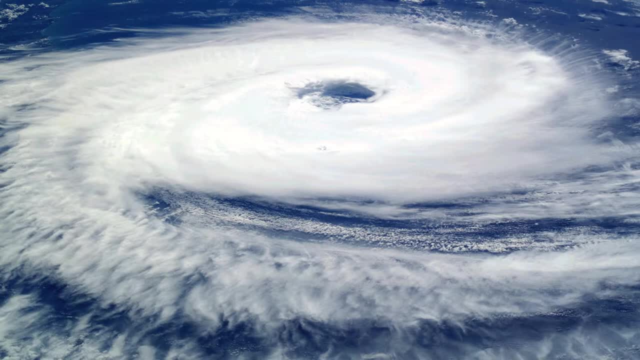 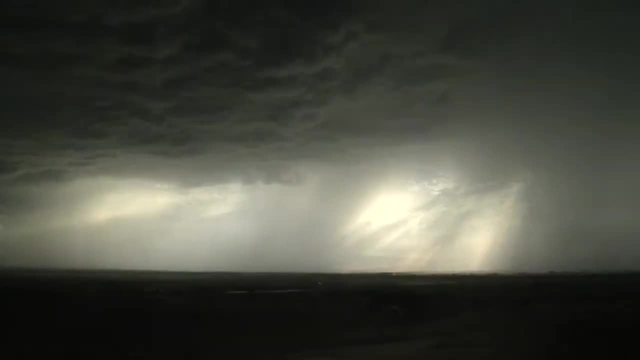 not just Pacific Ocean and islands, continents around Pacific, but also the whole global climate. Let's, in this video, talk about El Nino, how it's occurring, how it's related to La Nina, its effect on global climate and what we know about this phenomena from the 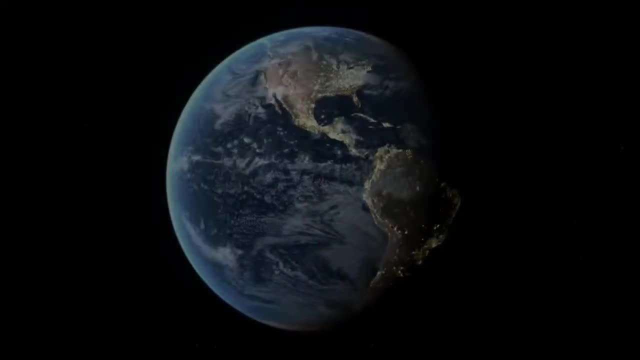 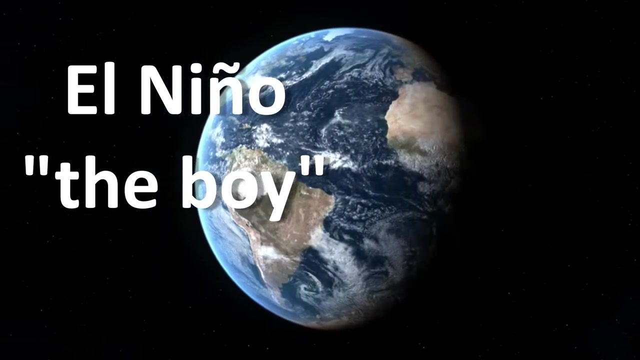 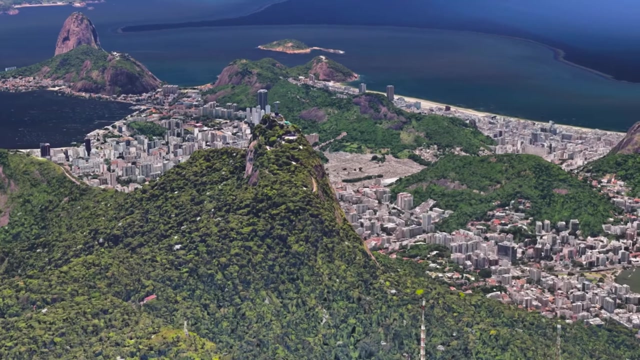 worldwide paleoclimatic record, One of the main effect El Nino traditionally had on South America. that's where the name come from. El Nino means the boy in Spanish. Traditionally it was called like that because the effect start been feeling around the South America. at the time of Christmas, Usually in El Nino years. the pool of warm water in the Pacific near South America is often as its warmest about Christmas. Back in the day, Peruvian fishermen named this weather phenomena after the Christ being born during the Christmas. 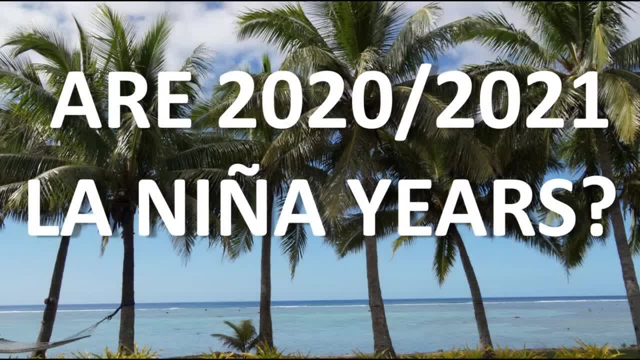 From my previous video, we learned that El Nino is the opposite or other side of Pacific oscillation, opposite to La Nina the girl. Watch my previous video about La Nina in 2020-2021, when I in detail describe what is ENSO El Nino- Southern Oscillation. 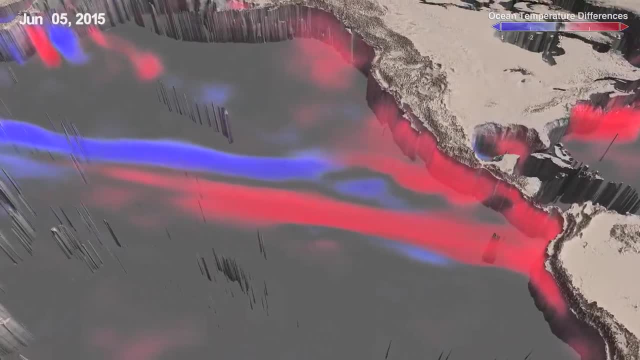 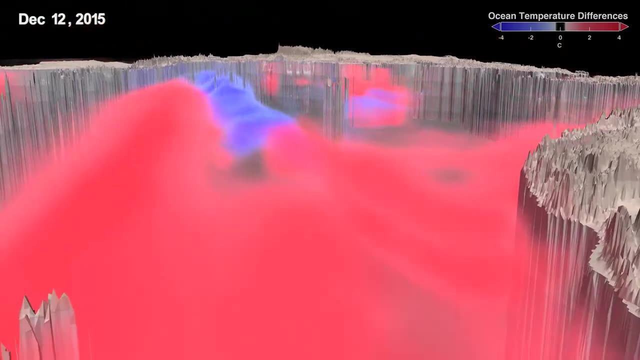 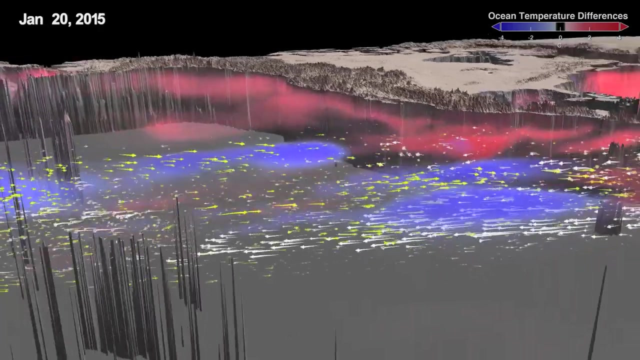 Briefly, it's the cycle of warm and cold sea surface temperature of the tropical, Central and Eastern Pacific Ocean. El Nino is followed by high air pressure in the Western Pacific and the lower air pressure in the Eastern Pacific, For example, towards Asia, Australia, New Zealand. we have high pressure Towards South. 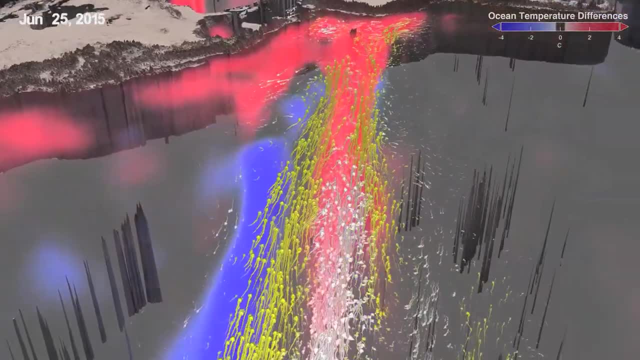 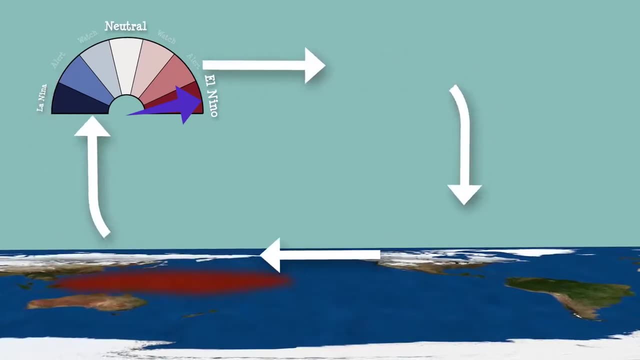 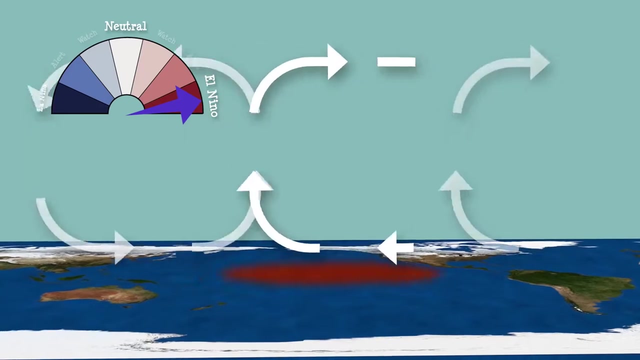 America, low pressure Phases of El Nino traditionally to be last from 2 till 7 years. However, from time to time, this El Nino effect could be different. Some El Nino years are stronger and have more global effect- catastrophic rainfalls or droughts- and some years, although it's happening, but in smoother way. We know that during the El Nino years, rainfall develops between September and November, And when it's opposite, we have the cool phase of ENSO, La Nina, the sea surface temperature in the Eastern Pacific below average and air. 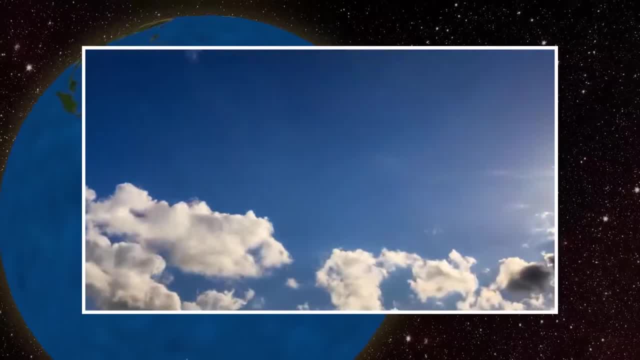 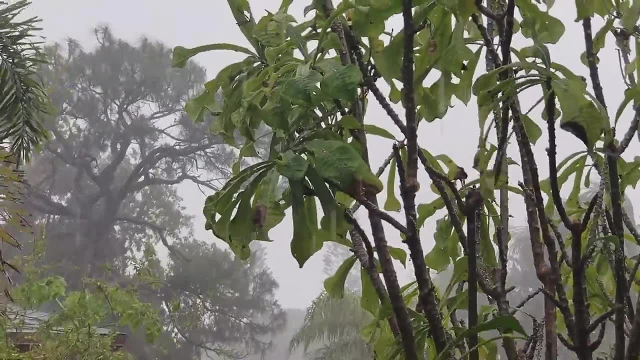 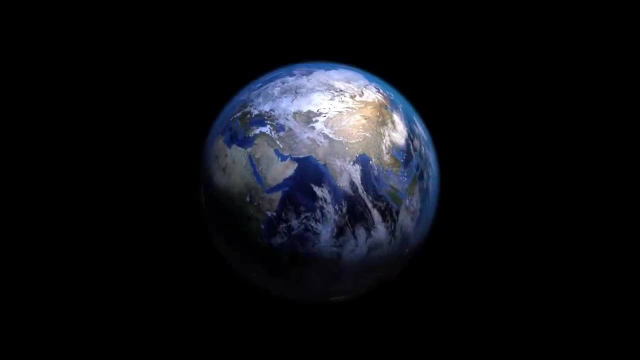 pressure high in the Eastern Pacific and low in the Western. Let's talk in detail how it's affecting the global climate and population which affected directly by these changes. Majority of developing countries are affected by El Nino or La Nina. We know that on our planet the climate is constantly changing, but we have the normal. 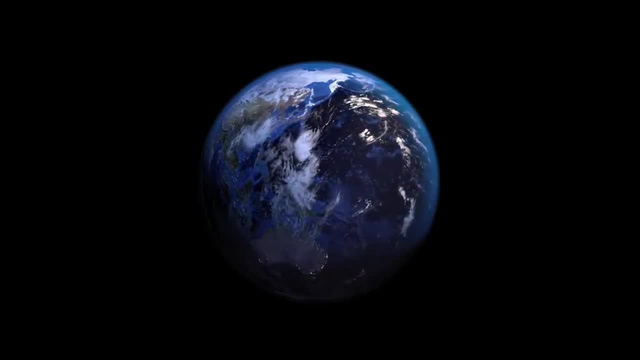 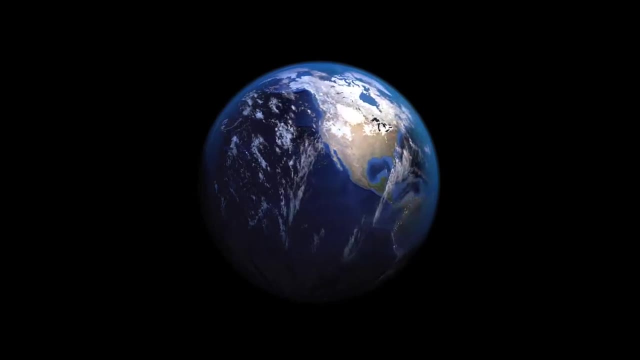 weather patterns, so more or less your usual average temperature through the summer, through the winter, how much precipitation falls in every of the season, and so on. However, we have very old years and in the climatology we know there's a different oscillation around. 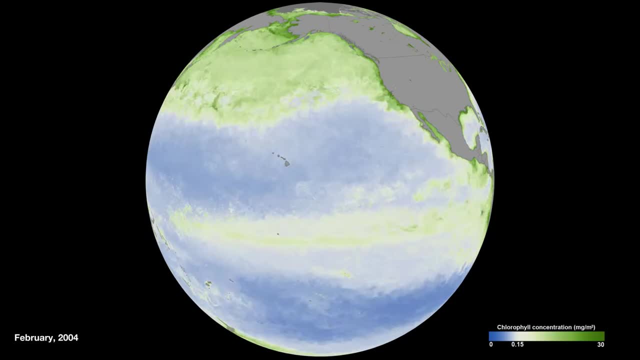 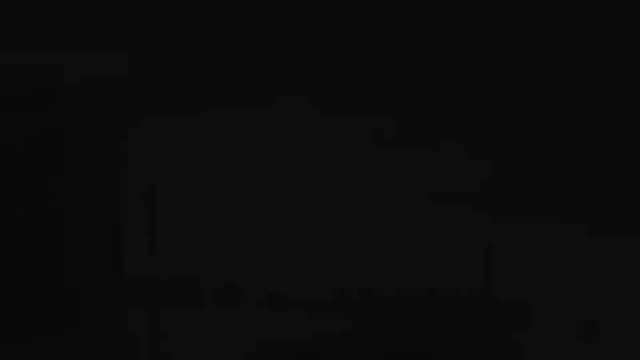 the ocean, interaction between ocean atmosphere, currents in the ocean which caused that, And one of the most famous one is El Nino- Southern Oscillation, one we talk about Because the Pacific Ocean is large and it's affecting the global climate dramatically. As a result, in the years of El Nino, we have this extreme. 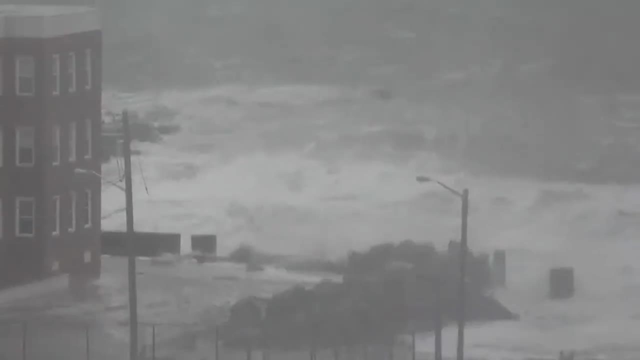 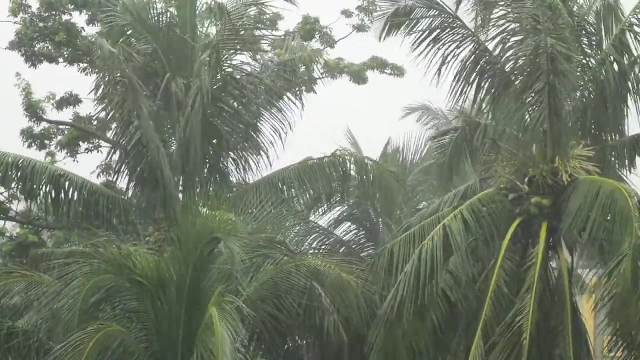 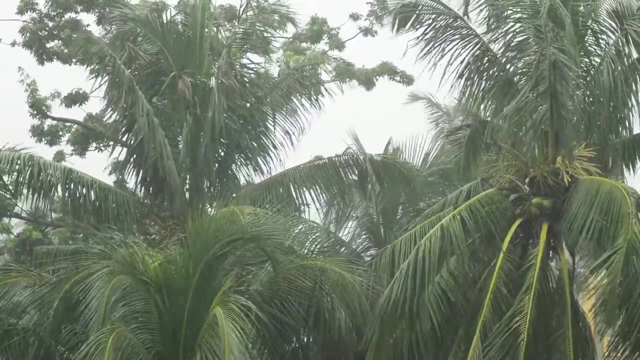 weather condition more common, Such things like intense storms in one places and drowns in some other places, And it will all depends on the regional exposition of the continents: mountains, streams, water and so on. One of the main effect that El Nino has on 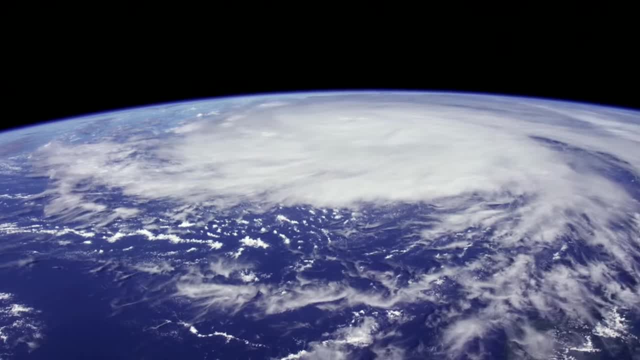 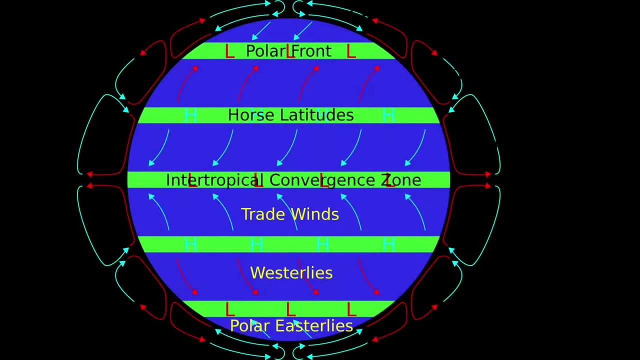 the global climate is on the tropical cyclones. Most of the tropical cyclones stay arising from subtropical and equatorial areas. Thus, for example, in Asia, in areas like Japan, Korea, these areas experience less tropical cyclones, developing in September till November in the years of El Nino. However, in Atlantic, 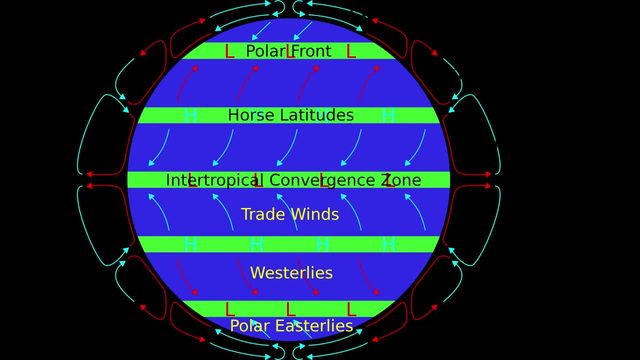 Ocean we see the opposite effect. This difference of the wind gradient increases and it's causing the western winds in the atmosphere to be stronger. At the same time, we know that the atmosphere over the Atlantic Ocean become a little bit drier than in the normal stable years. This difference in the gradient can cause the more 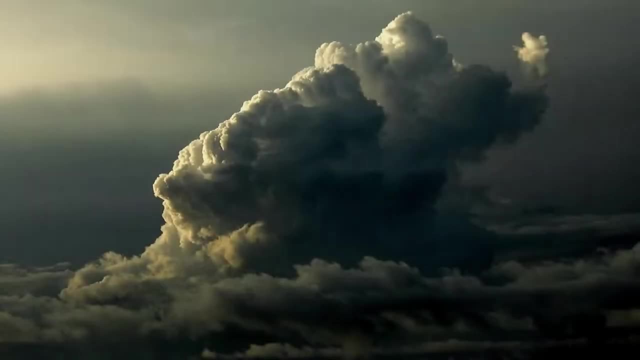 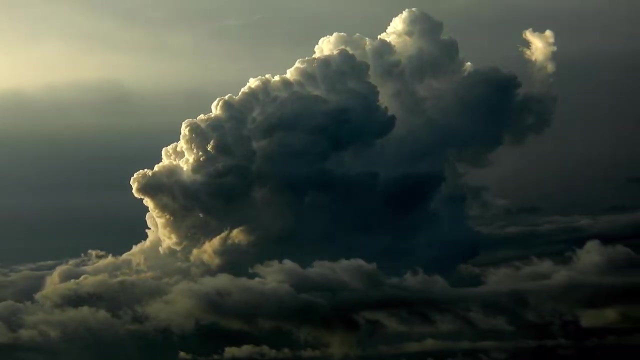 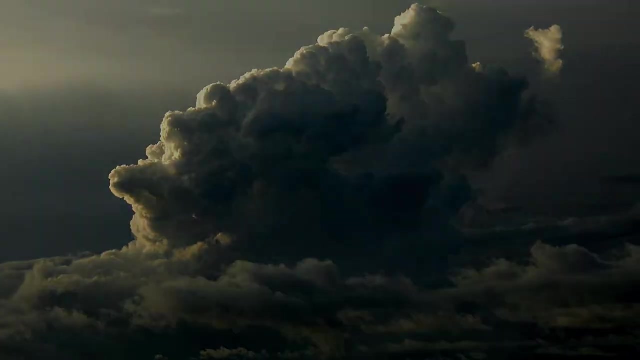 cyclones developing as well. Overall Western Pacific Basin tropical cyclones just a little bit changing the intensity and shift eastward. As a result, areas like Micronesia is more likely to be affected by tropical cyclones than China. In China, there's a less risk of cyclone activity. At the same time, in the Southern Pacific, tropical cyclones shifting as well, and it leaves the Australia region clearer. Therefore, tropical cyclones in areas like North and Eastern Australia dramatically reduce and increase the risk of cyclones falling down on islands like French Polynesia, Tongo, Tuvalu, Cook Islands and so on. 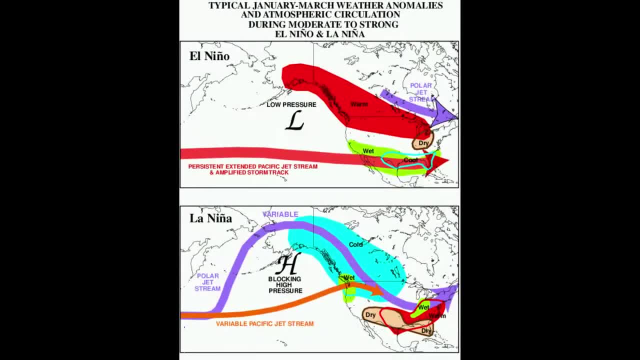 Closer to the eastern coast of America and Europe. we're noticing through the history that the North Atlantic have much warmer waters during the spring and summer, So you can see some changes in the weather in the northern Atlantic as well. For example, you can see the northern Atlantic have much warmer waters during the spring and summer. 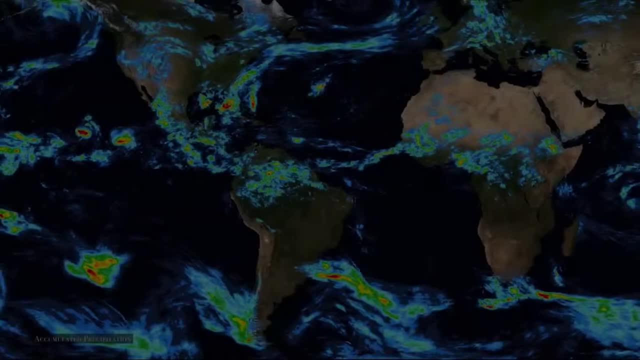 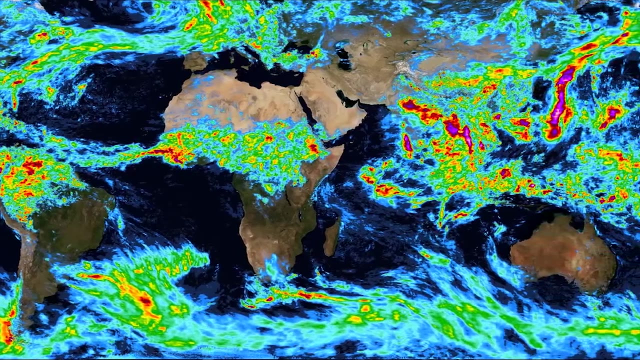 summer. However, in the eastern equatorial Atlantic we have unusual cooling events in spring and summer following the El Nino peak in winter. It's all related to El Nino effects on Atlantic water circulation over the South America that get strengthened in the eastern. 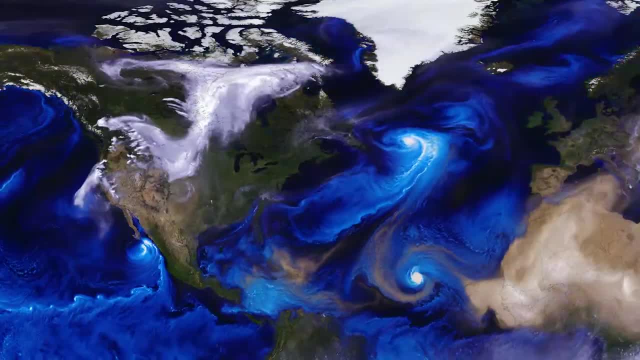 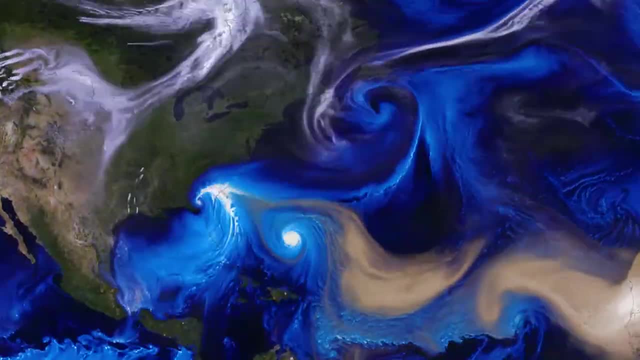 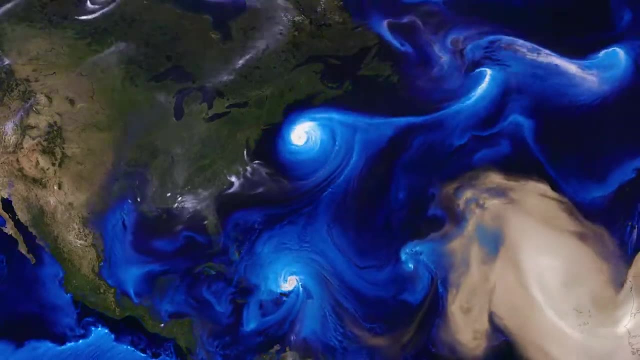 wind and western equatorial Atlantic region. Therefore, these El Nino-type years are affecting the population around the both oceans. We observe severe faintings which are a result of reduced monsoon rains. Let's closely look on the original effect of El Nino years. Just 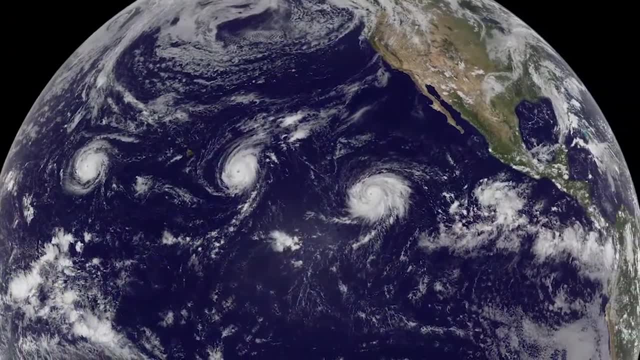 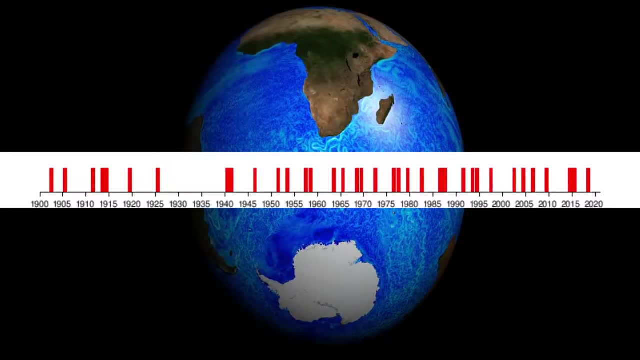 remind you, in my previous video, Le Nino, we looked on the original effect of Le Nino years, the one we experience right now. Let's talk about El Nino. We have direct observation of El Nino from the 1950s approximately and we have a long record of El Nino years from. 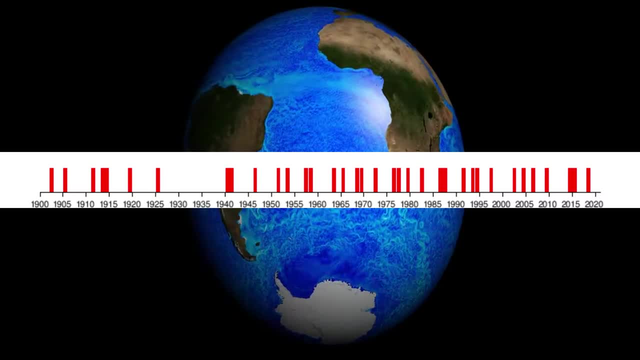 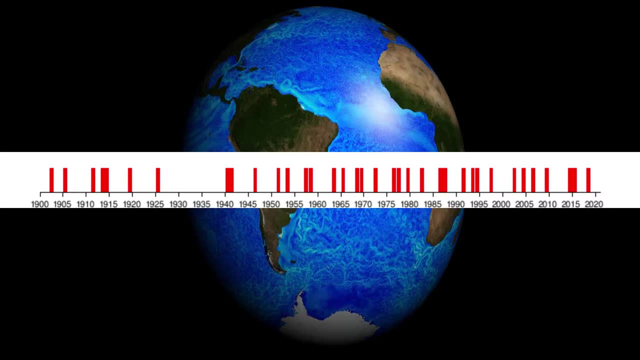 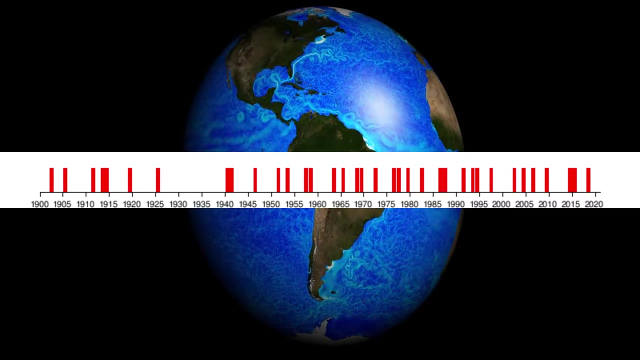 dendrochronology, tree rings from corals, ice cores and other paleoclimate data. However, you need to remember that each El Nino event, which occurs every 5-7 years, doesn't have to have the same original effect on the area. It depends on the background weather conditions. 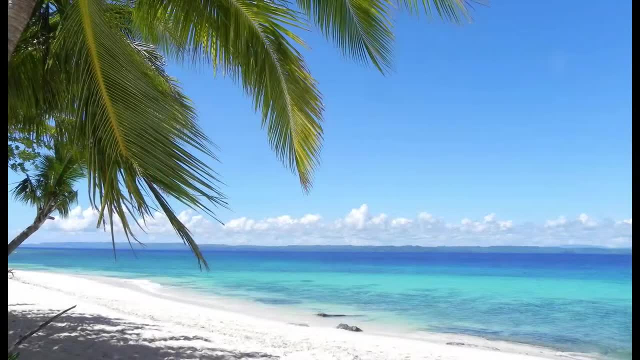 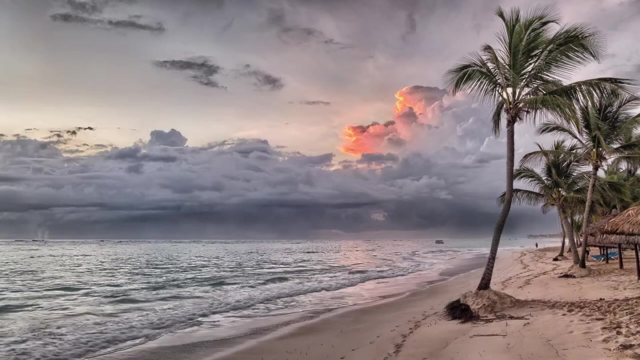 and the original situation at that time. However, we can draw the general picture of the impact of El Nino. For example, in areas like Indonesia and South America, we have reduced amount of the rainfall, while more the rainfall occurring in Southeastern South America, Eastern Equatorial Africa and the Southern United States. 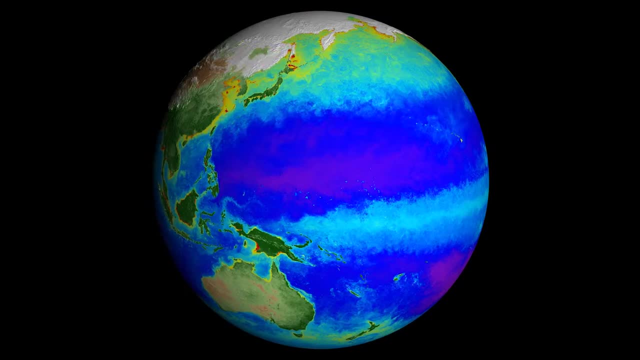 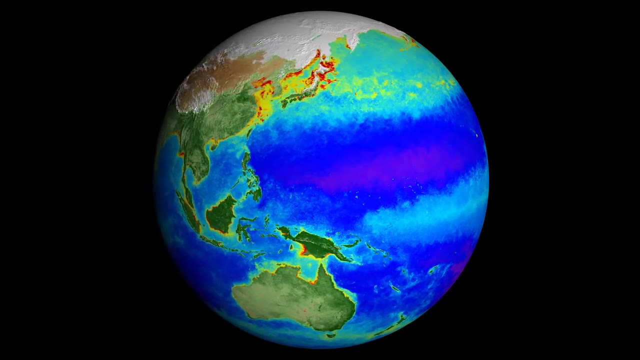 Let's consider Asia first. It's directly affected by El Nino. In El Nino years event, we observe a lot of warm water spreading from the Western Pacific and Indian Ocean to the East. As a result, we experience more drought in the Western Pacific and more rainfall in 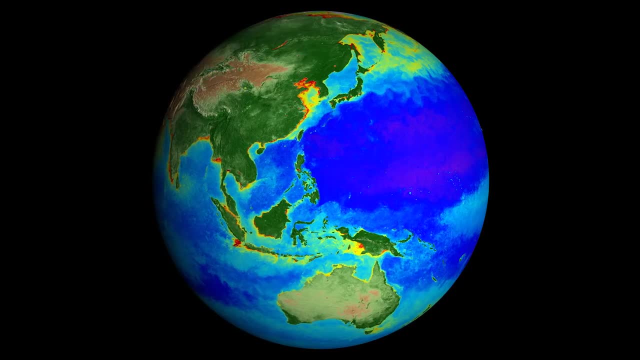 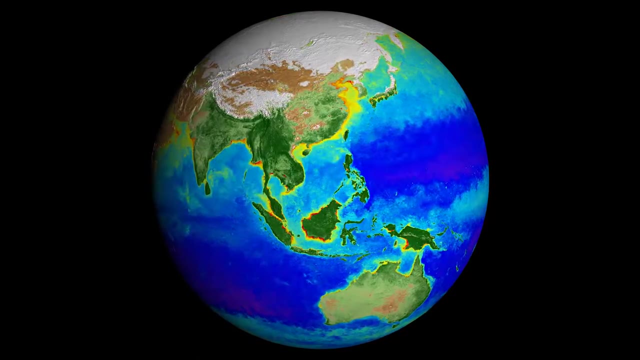 the Eastern Pacific. One of the driest years was observed in 1968, 2005,. 2014- years of El Nino. What about Australia and Southern Pacific? Here as well, because of the shifts of the rain eastwards, we have. 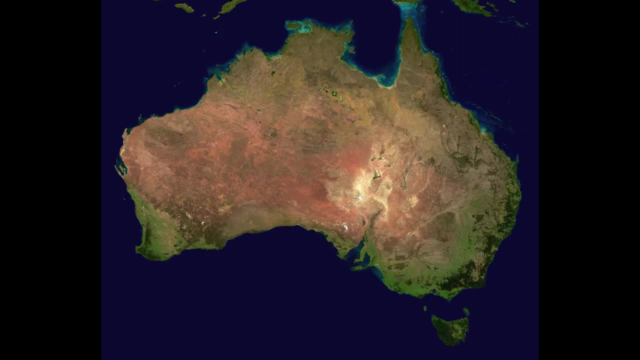 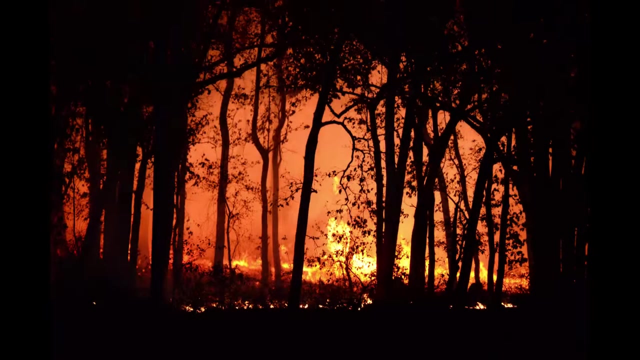 a drier area. We have warmer than average temperatures around Australia and very high pressure occurring. For Australia it's mean a lot of bushfires. This is the most famous and dramatic bushfires occurred in Australia. One of them, you remember, is the. 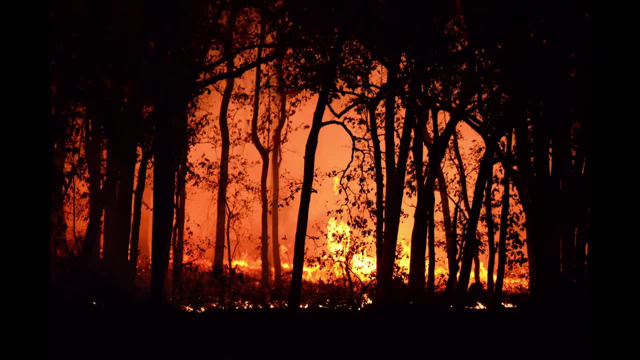 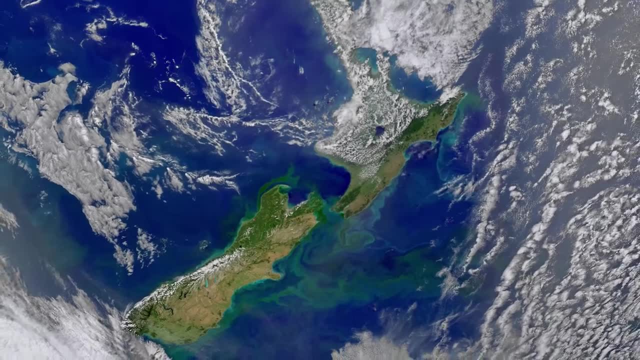 one that happened in the summer 2019-2020.. New Zealand affected directly by El Nino and experienced more frequent westerly winds during the summer. Therefore, there's a much more drier condition in New Zealand that time. However, in areas like west coast of. 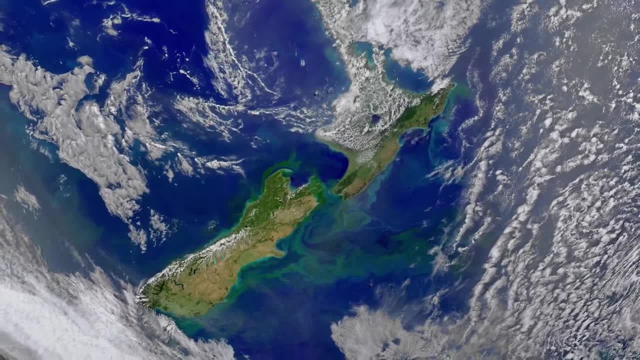 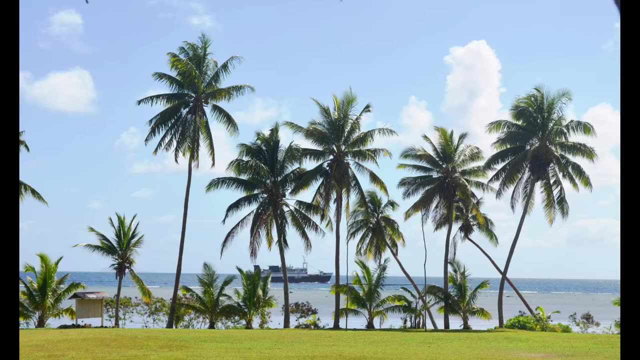 the Southern Island experienced more rainfall. abroad from the west Islands around the Pacific experience dry and abnormal conditions, such as in Fiji, and can lead to the drought as well. The sea surface temperature can cause the bleaching of the corals which have a big 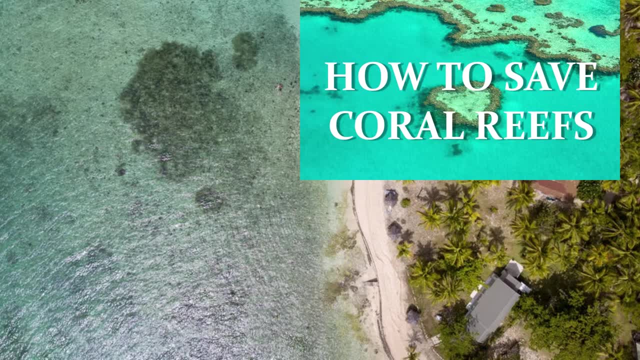 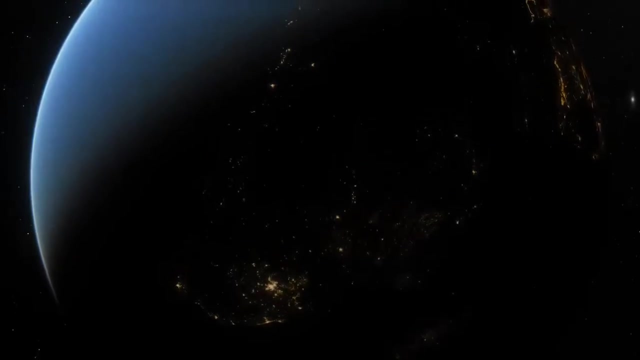 impact on population, with dying corals, the fishes and all the life around the islands dying as well, And this also have effect on next tropical cyclones destroying the islands easier and faster. Watch my video about coral reefs. Let's talk about Africa. Africa is affected by El Nino as well, like we talked before. 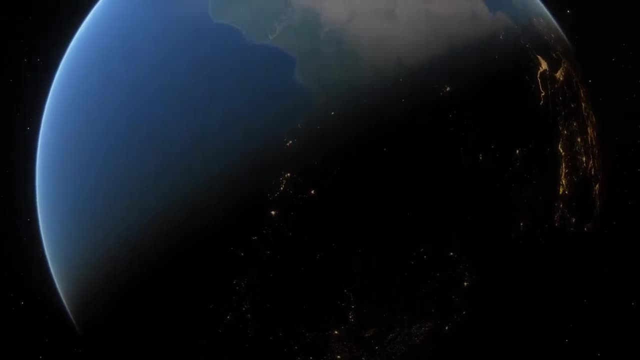 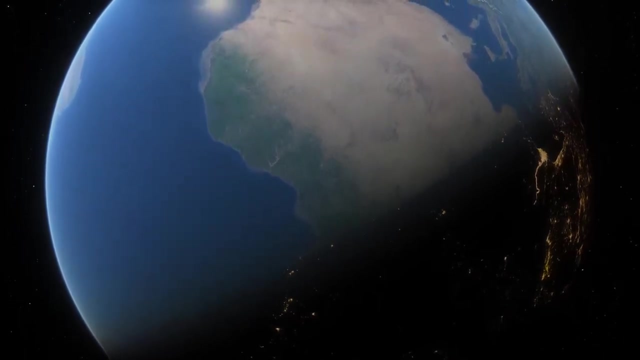 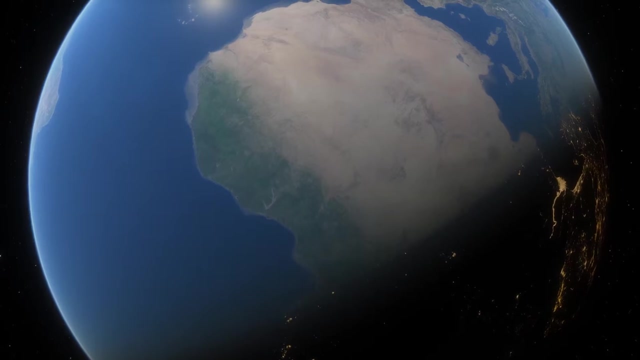 by Leonino. In the areas east of Africa, including Tanzania, Kenya and so on, we experience long rains from March to May. However, dry conditions than normal are observed in South Central Africa countries like Zimbabwe, Mozambique, Zambia and Botswana. Scientists reporting. 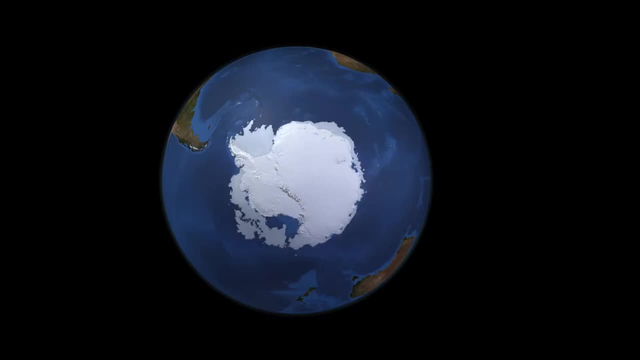 the effect of El Nino on the sea surface, including the southern Gulf of the Pacific. El Nino on Antarctica: We notice the high pressure developing over the parts of Antarctica, which reduces the sea ice and increases poleward heat fluxes in these sectors. We know the 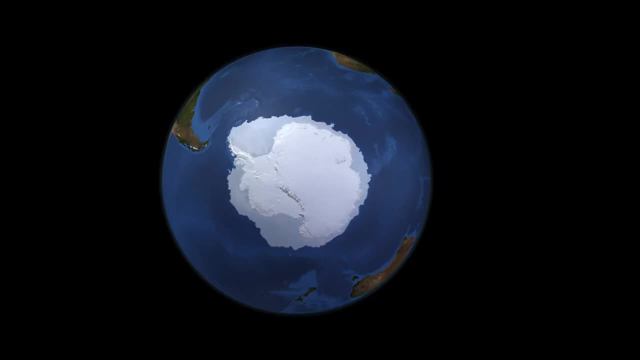 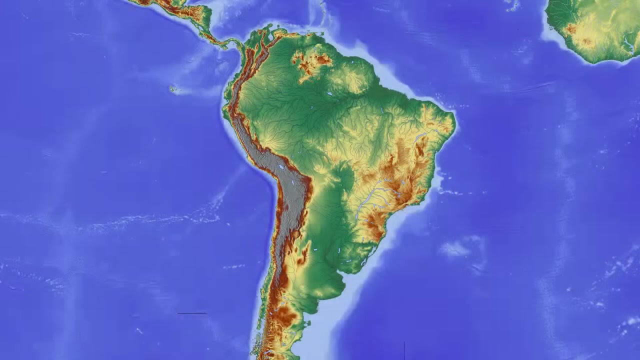 absolutely opposite effect during the El Nino. We call these patterns an Antarctic Depot mode. Let's talk about South America. South America is dramatically affected by the El Nino and from the name we figure out. that's where people first start naming this phenomenon. 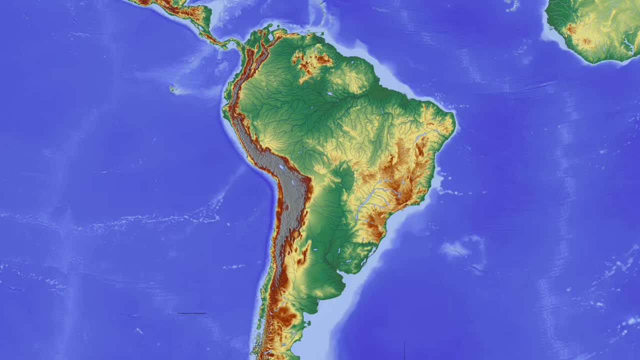 We already said that all around South America we have increase of rainfall and it's also the effect of it much more pronounced than in North America. In April to October you experience quite a wet weather. around Peru, Ecuador, They're also very common, the extreme. 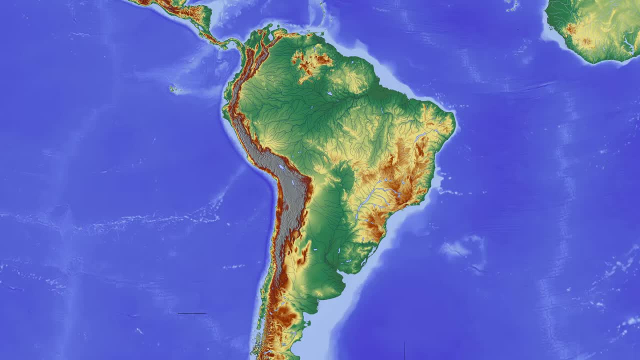 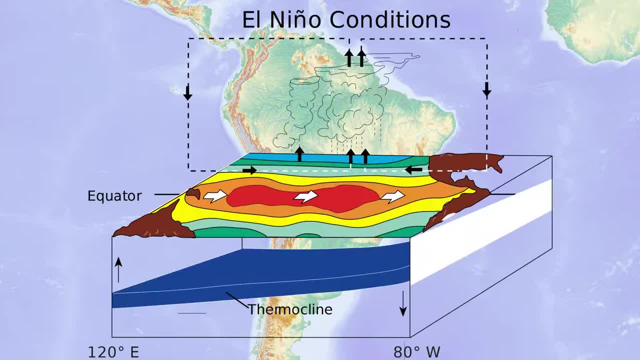 The main general effect which El Nino has become the obvious in February-March and April. The main general effect which El Nino has become the obvious in February-March and April: El Nino reduces the upwelling of cold, nutrition-rich waters from the bottom of the ocean. 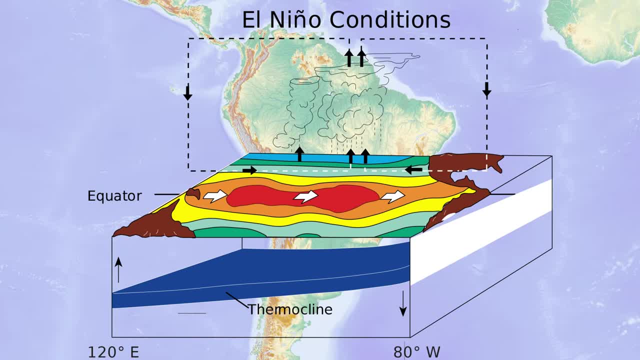 and therefore the all marine life- fish population, birds and so on- reduces dramatically. It's affecting the fishing industry in that area and sometimes it's even caused catastrophic economical problem. Farther south of South America we also experience much wetter condition than normal, usually in spring and early summer. However, you can expect it that 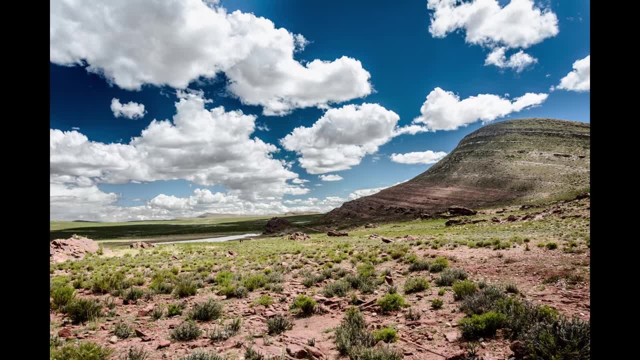 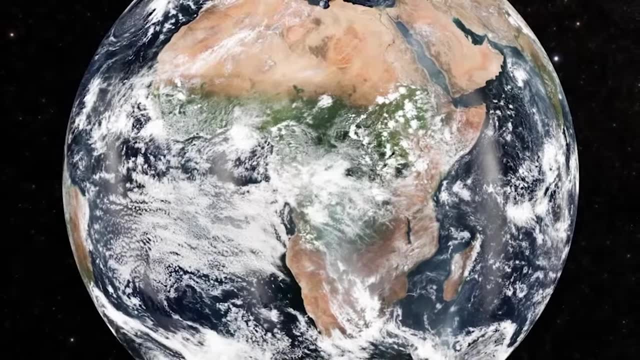 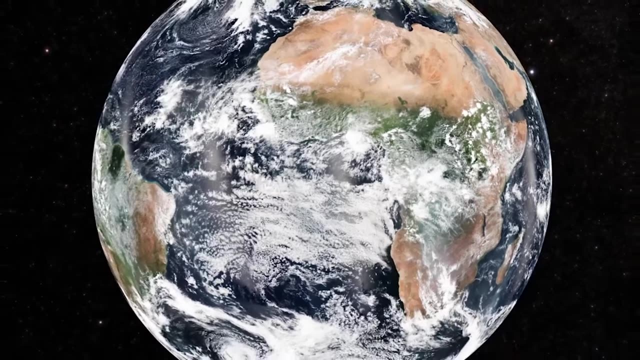 drier and hotter weather occurring eastward from the Andes, around the Amazon river basin, Colombia and Central America. Therefore, these years of extremes- El Nino or La Nino- they affect not just the regional weather patterns but also the economy of this area. 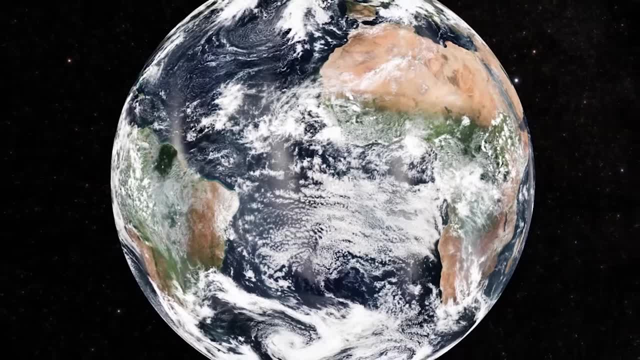 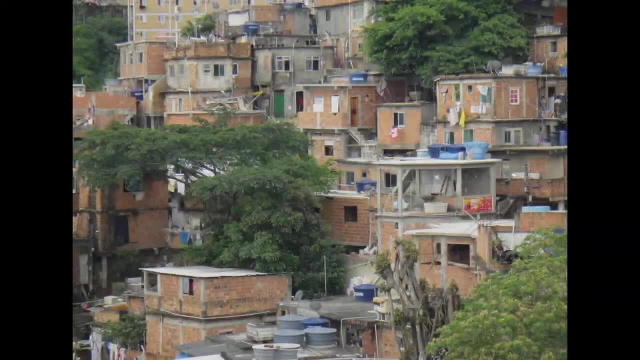 population. they have social impact, health impact and it's also affecting ecology, as we already mentioned before, And specifically El Nino is quite effective on economy directly in South America. by reduced upwelling we have dramatic effect on fishing industries. 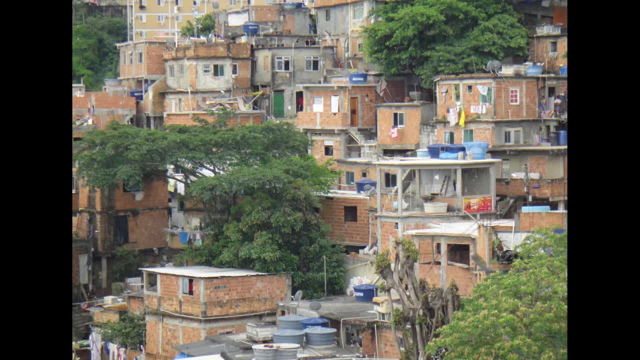 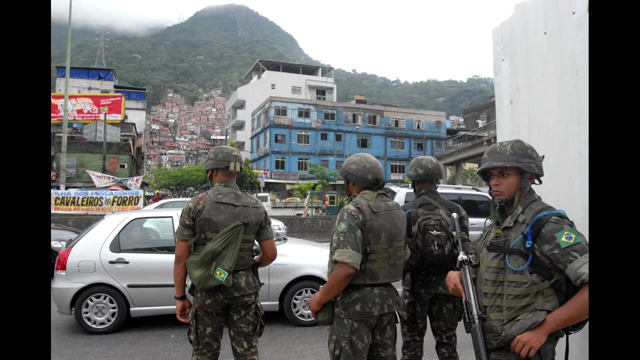 oil prices increasing, international interactions decreasing and it's caused extra pressure on the population economy. Scientists reporting that a lot of health effect pandemic developing during the El Nino years could be caused by particular disease transmitted by animals or just by the particular weather condition: floods and so on. From the ecological consequences, 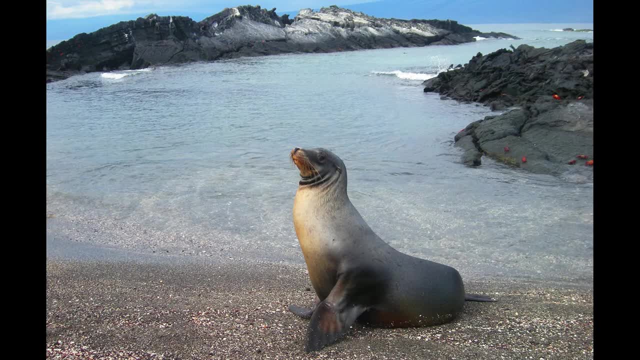 the El Nino will affect the marine production, the animals living in the sea, birds and mammals. In areas when we experience a lot of dry periods, there'll be dramatic effect of bushfires on the forests and animals there And for the ocean all these oscillations have 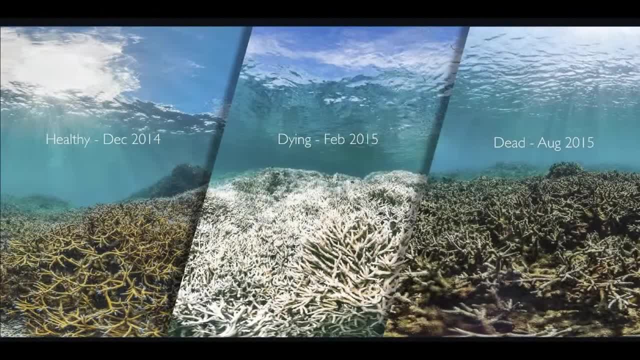 dramatic effect. as we talked about the corals, the global moth bleaching events occurring there. One of the most important and severe was in 2015-16, when we recorded more than 70% corals loss around the world. This is due to the increase in the number of corals in the 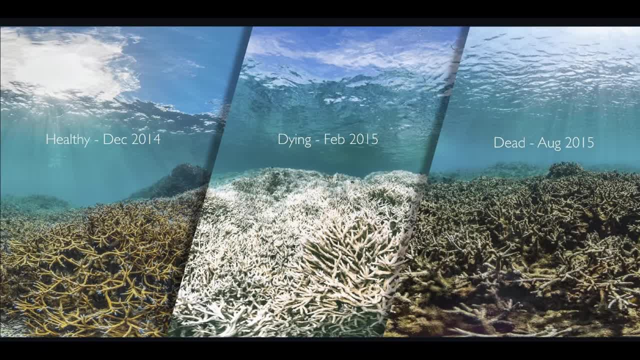 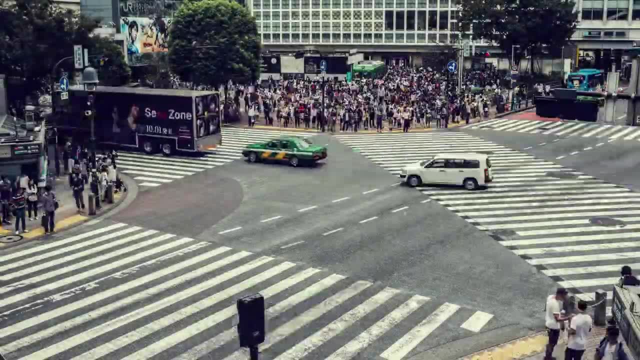 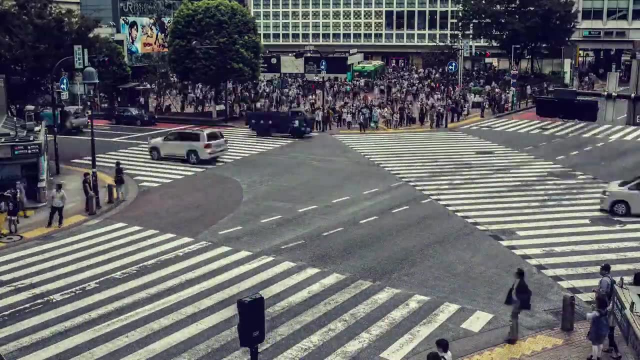 world, Therefore, biodiversity on our planet around Pacific, and not only affected by these events, But what we people can do to help during the such events to our planet to strive and survive. For that we need to understand how El Nino-La Nino oscillations works, Why, How they. 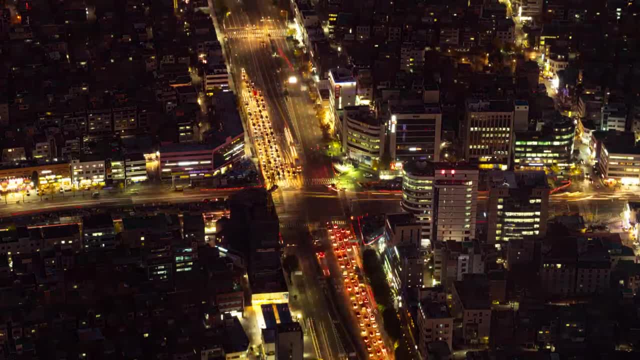 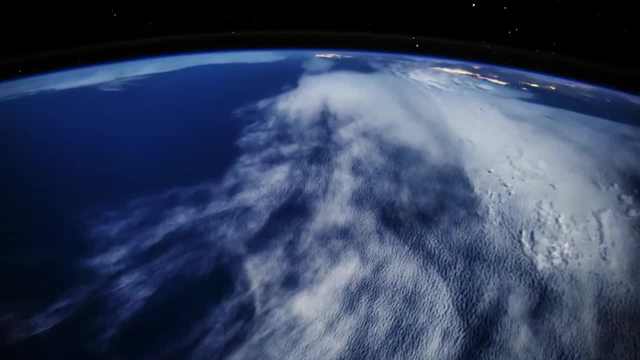 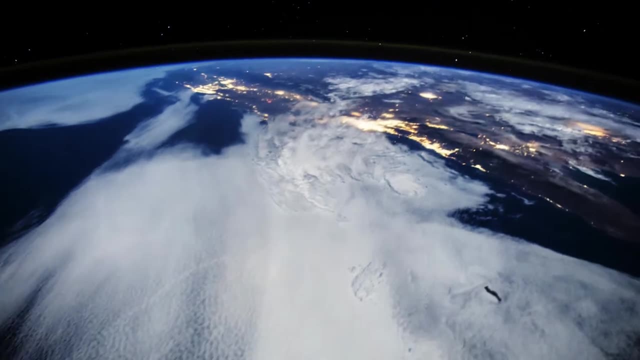 become more intensive and severe. Is there any impact from our activity on it? We will investigate more about periodically of these events: when they started and, more important, why they occur on our planet. what modern scientists think about that. One of the things you can do right now to help our planet is to subscribe to my channel and put like. 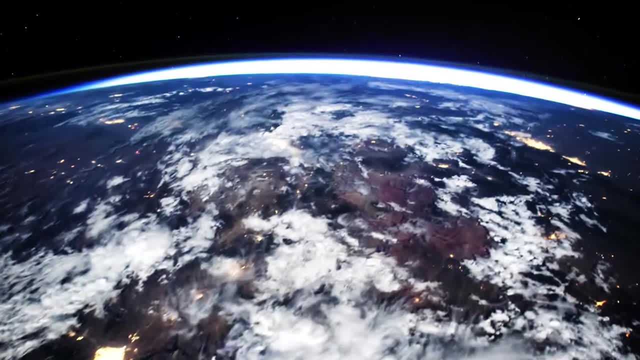 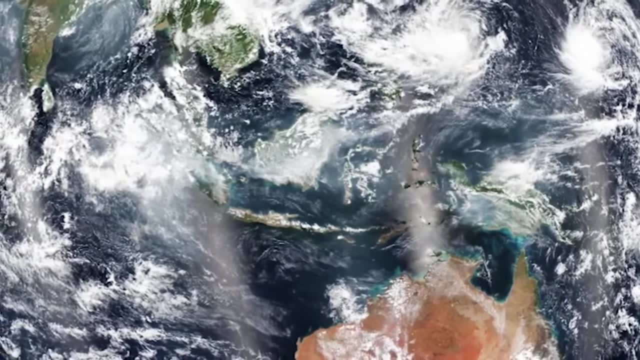 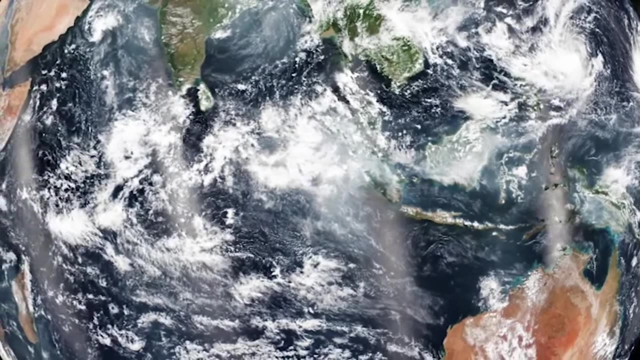 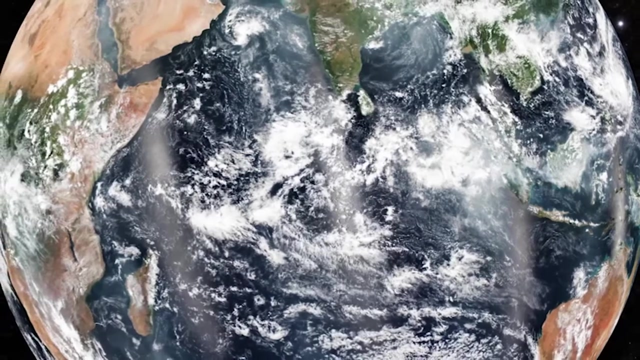 on this video. I'll see you in the next video when we explore more the secrets of our planet. Thank you for watching and see you in the next video.